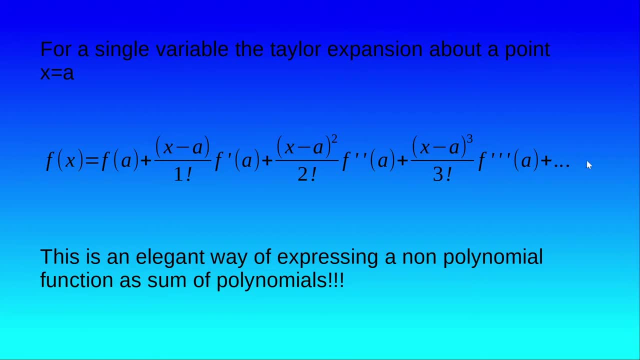 differential. Now this is the expansion of Taylor series of the function at a point a. This is a very elegant way of expressing a non-polynomial function as a sum of polynomials. Now, this is the beauty of Taylor series. Now let us look into what would be a non-polynomial function. 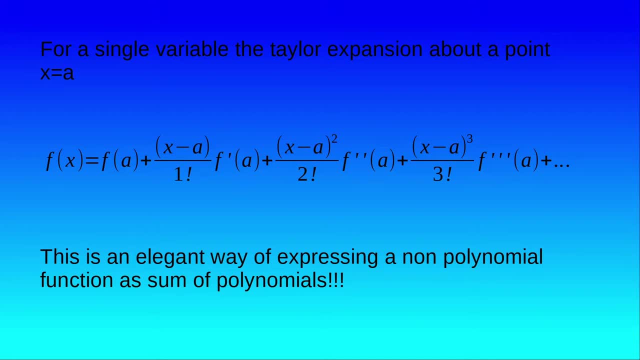 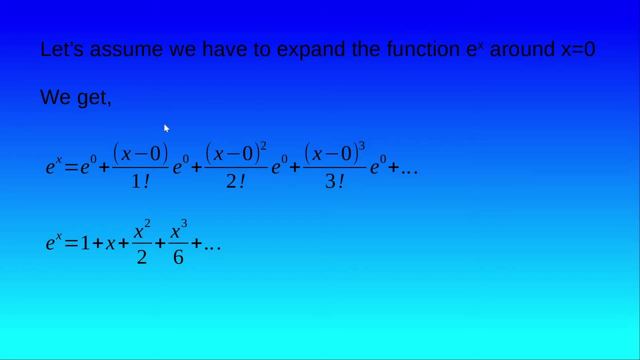 Let us assume we have to expand a function. e raised to x around x is equal to zero. Therefore, we get e raised to x as this: e raised to zero plus x minus zero over one factorial e raised to zero, x minus zero square over two factorial e raised to zero plus x minus. 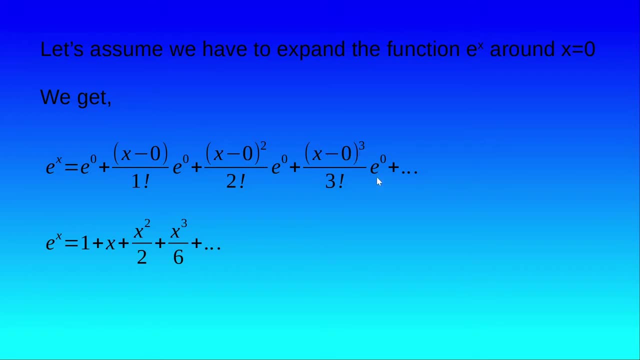 three x minus zero, the whole cube multiplied by three factorial, multiplied by the first differential of the function at a plus x minus a times x minus zero, multiplied by the first e raised to 0, and so on. so the expansion will result in this expression. now, if we take it to, 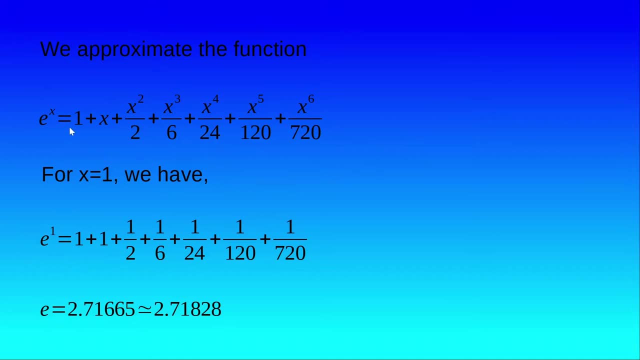 the first five terms, it would look like this: 1 plus x plus x, square by 2 plus x cube by 6 plus x, raised to 4 by 24. mind you, this is 2 factorial. this is 3 factorial. this is 4 factorial 5. 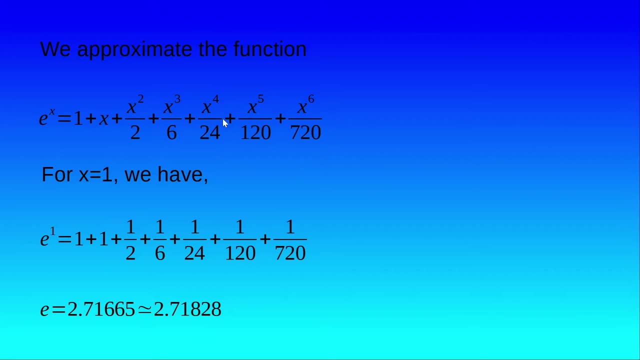 factorial, 6 factorial, and this is x raised to 6, x raised to 5. now let's estimate e raised to 1. so for x is equal to 1. we have this as the series. now this gives you a value of 2.71665. 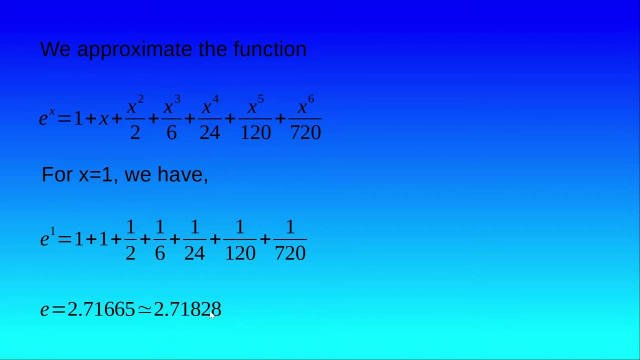 which is very, very close to 2.71828, which we have found using the calculator. so now let's have a look at the next one. look at what would be the truncation errors. it is best if we look at what is truncation errors using a spreadsheet. the idea would be a bit more clearer if we would actually speak about it. 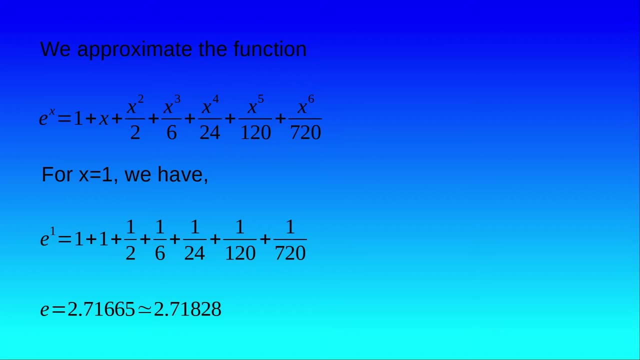 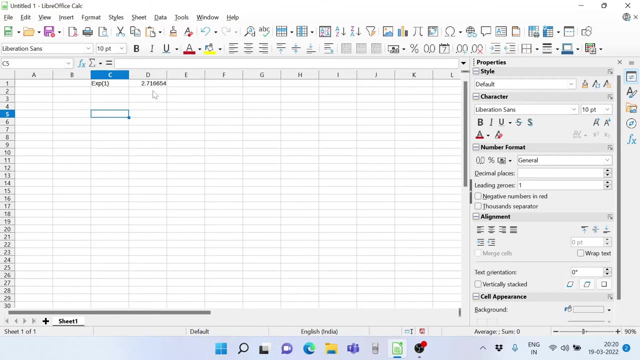 rather than we calculate it on the spreadsheet and demonstrate what are truncation errors. so this is the spreadsheet, or where we can study the truncation errors. so let's write the terms first: one, two, three, four, five. so in the first term we have one. in the second term we have one, Oh, one, factorial. so let us calculate the factorials. 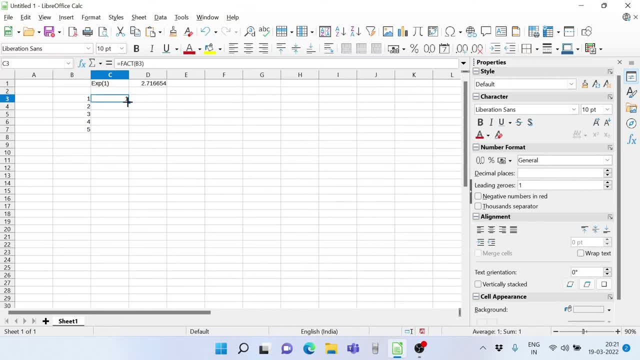 of these numbers. now, the terms should not be as long an interval as 15 seconds. so this is the depending on your foundation terms. Have you learnt the limits terms are: the first term is nothing but 1 divided by 1 factorial. 1 divided by 1 factorial. 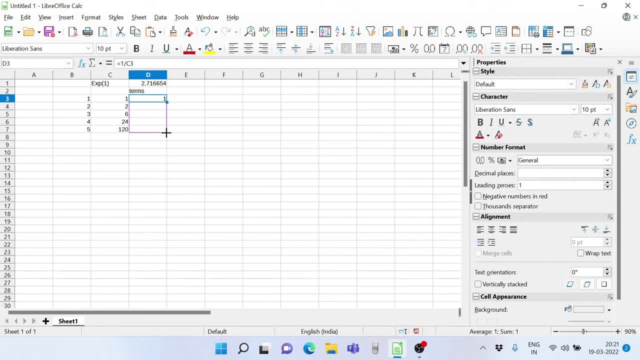 that is it. and similarly, we calculate all the terms. Now the final value of the function is equal to 1 plus the sum of all the terms. So these are all our terms. So there we have. If we take the sum of all the terms and add 1 to it, we get the. 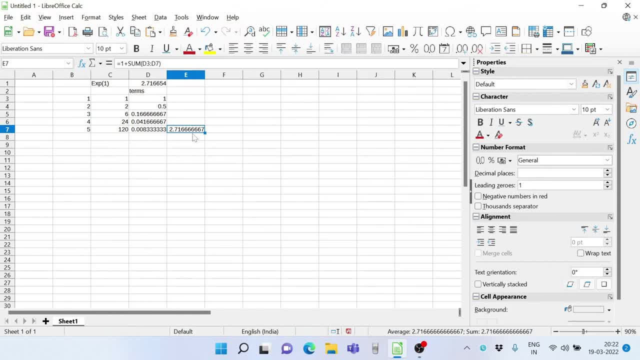 estimate as per the equation that we have just given, or just derived, for calculating exponential of x. Now what if we calculated the value of the exponential only using the first term? How much would be its value? So it would be 1 plus the first term. 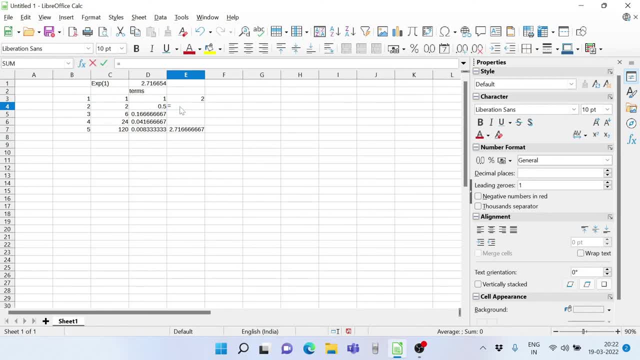 Now what if we calculate the value using the first two terms? So it would be the previous term plus the second term, and let's do it. This would be the value for the third term, and this would be the value for the fourth term. Now the truncation error. 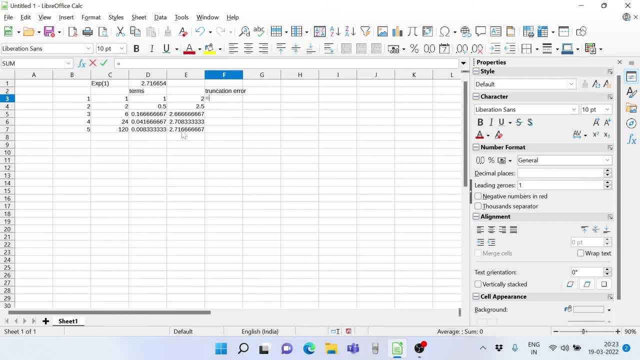 is going to be equal to the value that we have minus. that is the value that we have calculated using the entire expression with five terms, minus the value we calculate using the term. So this is the value or this is the truncation error that we are going to have, in case. 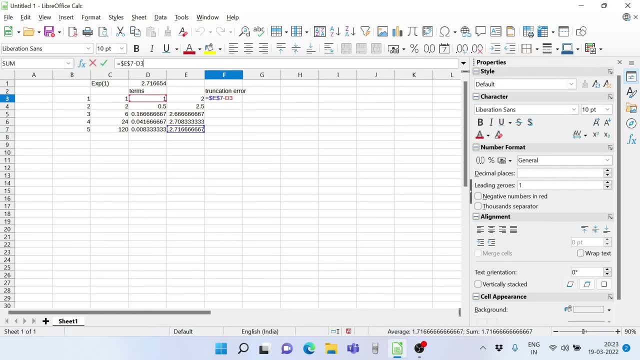 A slight mistake here, let me. yes, this is the value of the function. Yeah, So this is the truncation error we are going to have in case we take only one term, And this is the truncation error in case we take two terms. 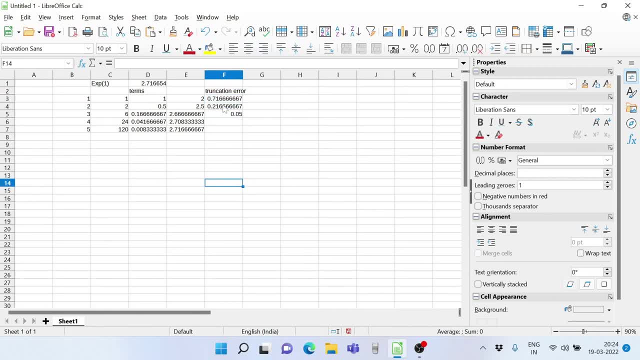 Now, this is going to be the truncation error, in case we take three terms. So what is this exactly? This is nothing but the value that we have calculated, value that we have calculated using the expression minus the value we have calculated using only the. 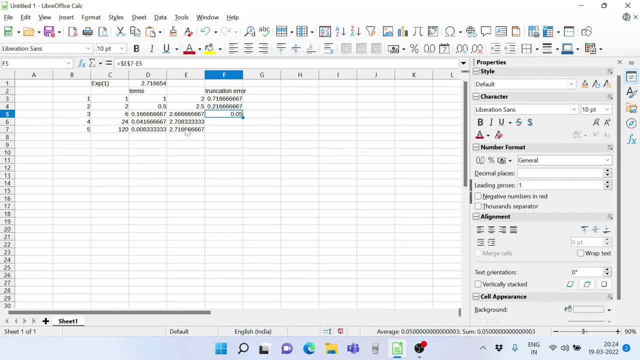 first three terms. now the difference of this and this is nothing but the truncation error. now, what does truncation mean? truncation means neglecting higher terms. now let's take an example. we have an expression in which we have five, ten terms. if we say it has been truncated, 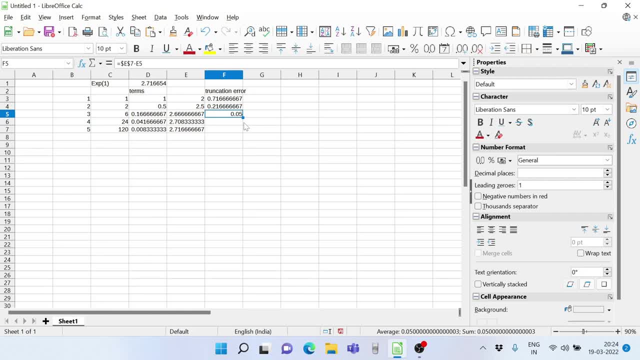 okay, from the sixth term it means 6, 7, 8, 9, 10 terms. 6, 7, 8, 9, 10 have been neglected. if we say we have truncated from the third term, then we say from the third term to the 10th term. 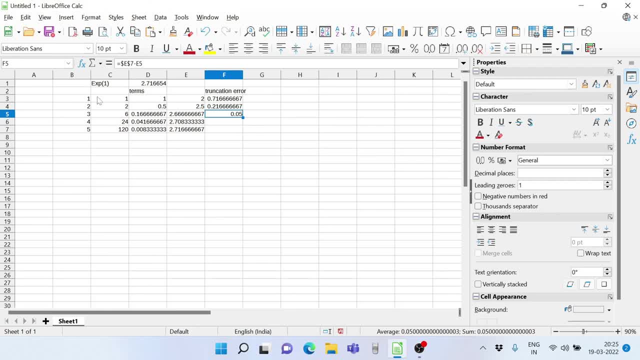 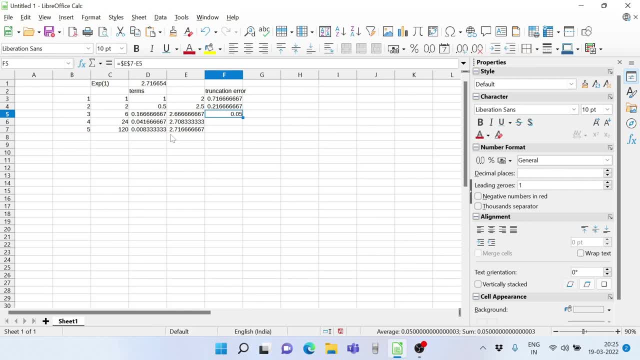 a fairly accurate value which was very close to that we have done in the calculator. So this is all about truncation error. So this is the truncation error we get using first four terms. So hope you have understood what is truncation error and do like and subscribe.